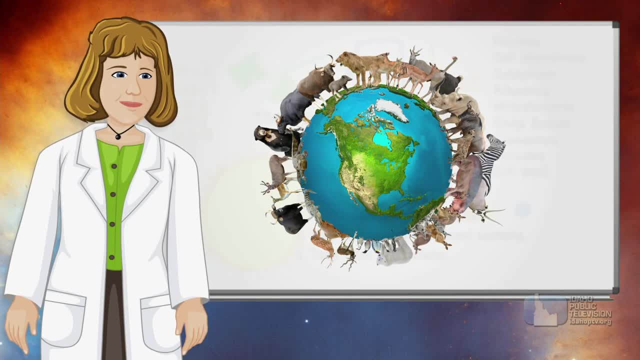 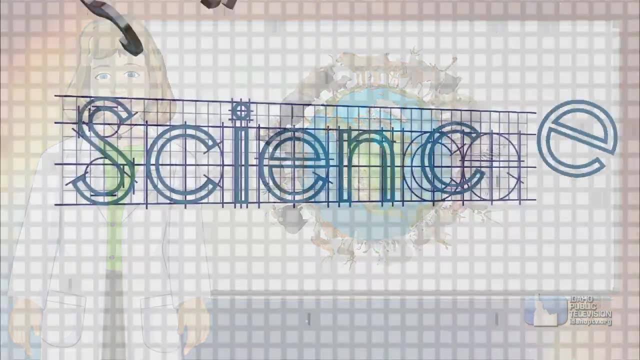 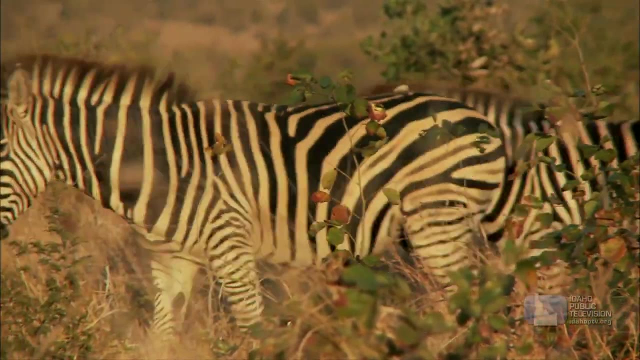 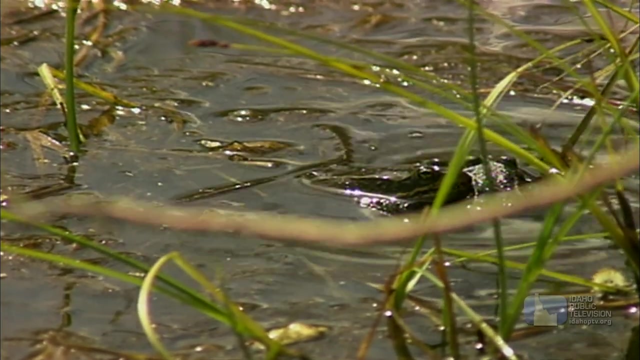 The number of endangered species in our world is pretty frightening, but there are folks out there trying to make a difference. Find out more about endangered species. The news about endangered species is not good. One in four mammals, one in eight birds, one-third of all amphibians. 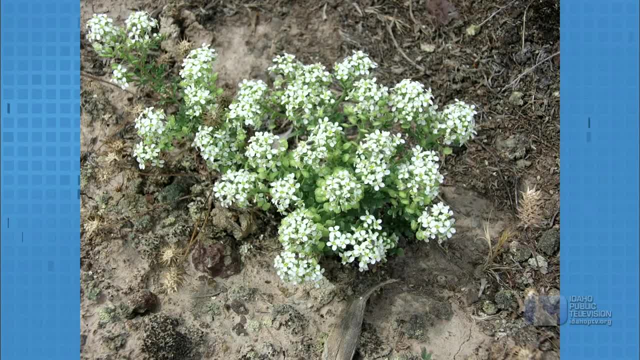 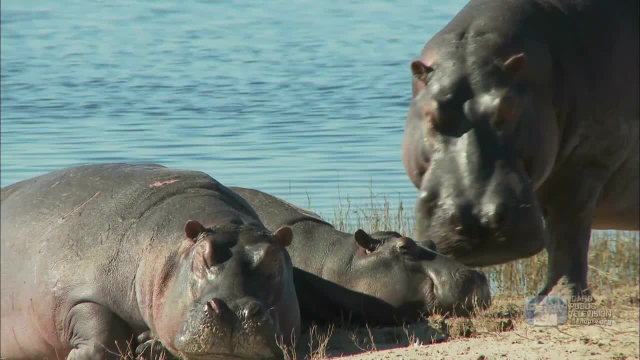 and 70% of the world's known plants are in danger of extinction. A species is in danger when the number of that species drops by more than 50% over 10 years, or if there aren't enough adults to really increase the population. 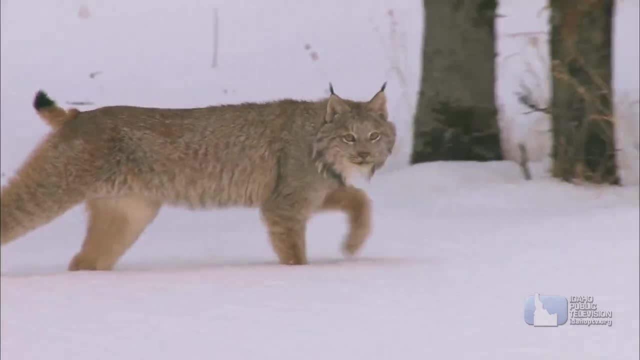 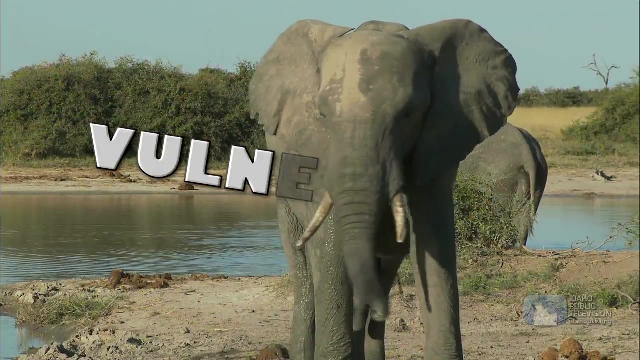 or if there isn't enough habitat to keep the population alive. Scientists define the level of threat to the survival of a species in four ways: Vulnerable A species is defined or classified as vulnerable when it faces the loss of its habitat or from threats like poaching. 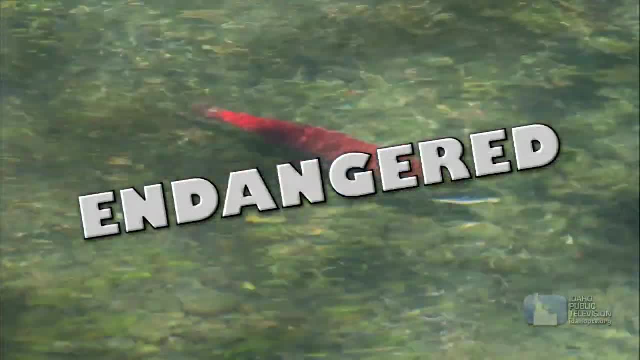 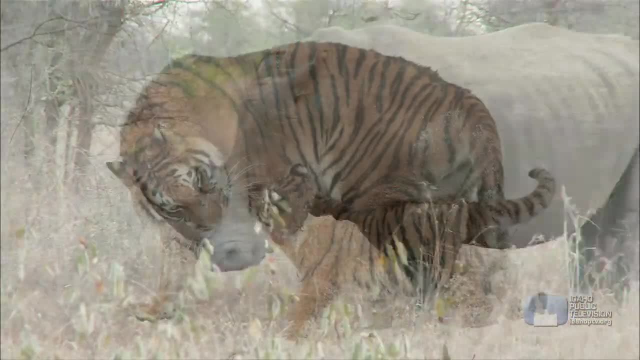 Endangered. A species is classified as endangered when the population of that animal or plant is dangerously low or when its habitat is disappearing because of pollution or human activity. Critically endangered A species is critically endangered when few of that plant or animal exist in the wild. when there are so few left that they may not be able to find a mate or produce young. And finally, there is extinction. A species is extinct when there are no animals no more left, either in the wild or in captivity. In the last 500 years, over 800 species have gone extinct. 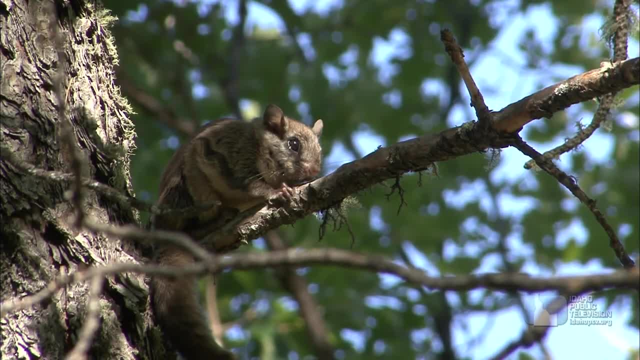 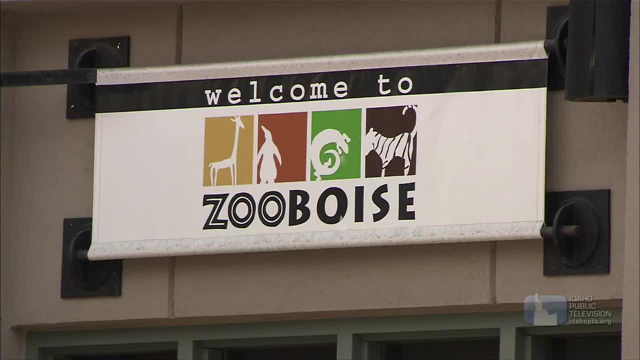 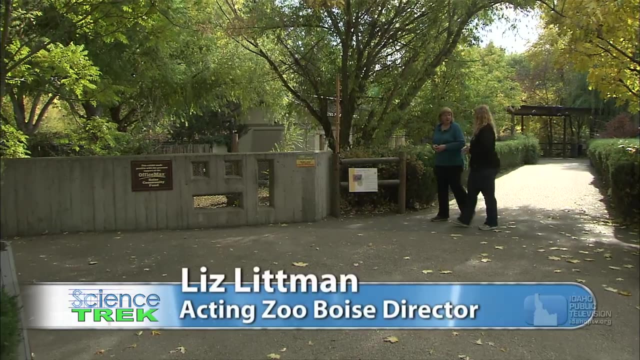 But now we're seeing the extinction rate increasing 1,000 to 10,000 times past rates. Dozens of plants and animals are going extinct every day, But places like Zoo Boise and its staff are doing their part to save animals. Well, we think it's really important to not just protect the animals that we have here in the zoo. 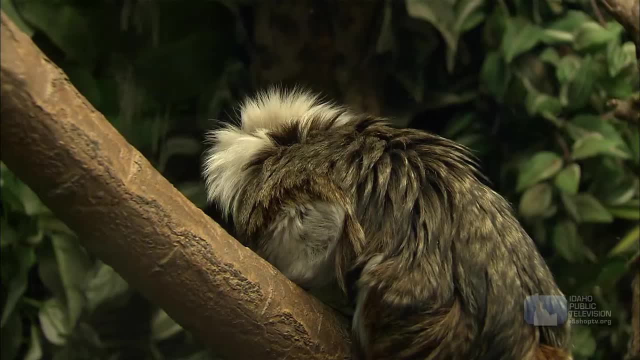 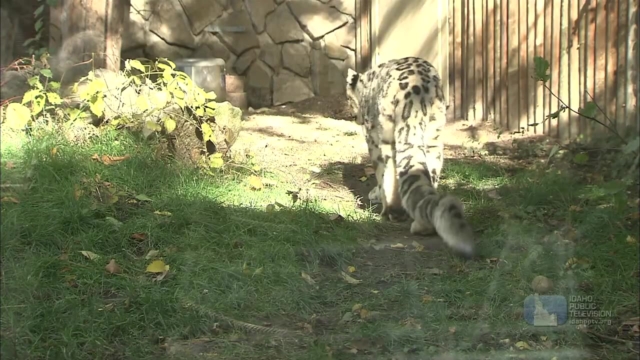 and take really good care of them, but to protect their counterparts out in the wild. Zoo Boise is home to more than 100 different animals. 24 are classified as vulnerable, endangered or critically endangered. These are our Vizayan warty pigs. 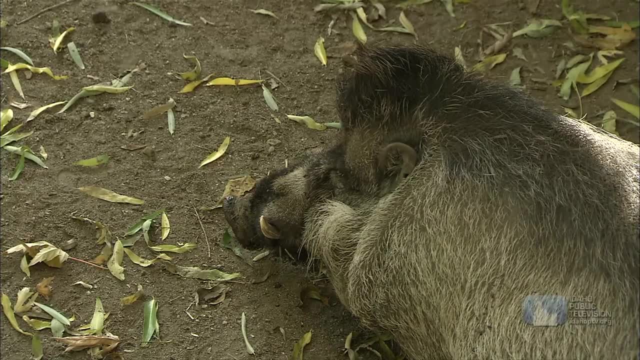 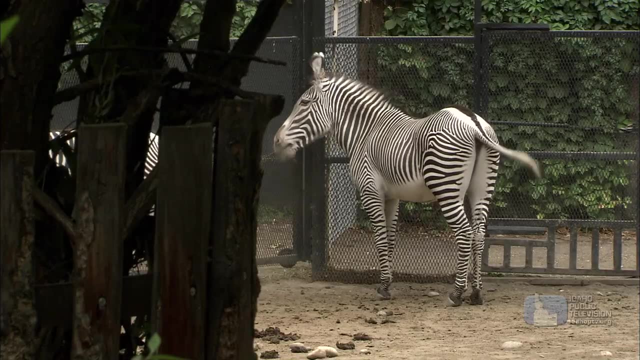 They are a native pig species to the Philippines and they are also critically endangered. At one point they were native to six islands of the Philippines and have already gone extinct on four of them. This is one of our Grevy's zebra. 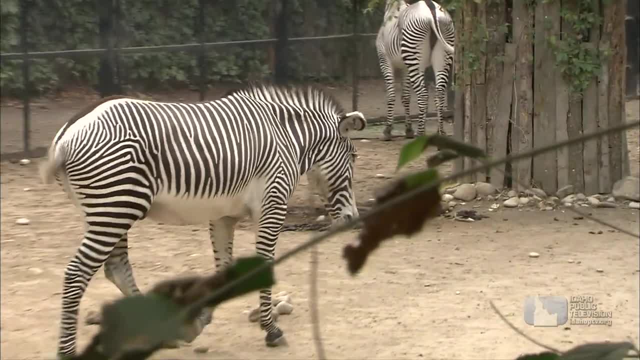 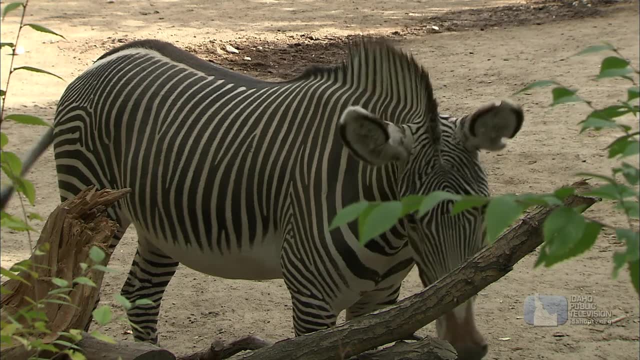 They are a subspecies of zebra native to Ethiopia and Kenya and Somalia And they are also endangered And that is mostly due to the habitat loss. Grevy's zebras. you'll see they have a different stripe pattern than other zebras. 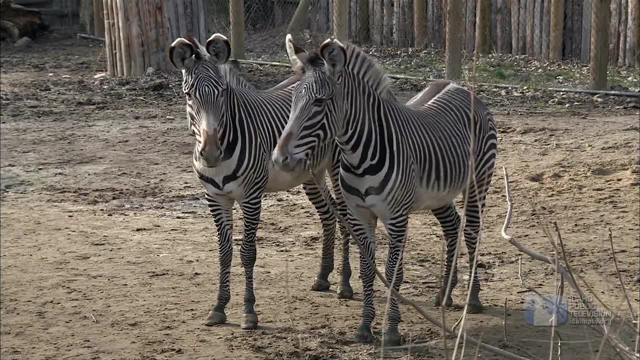 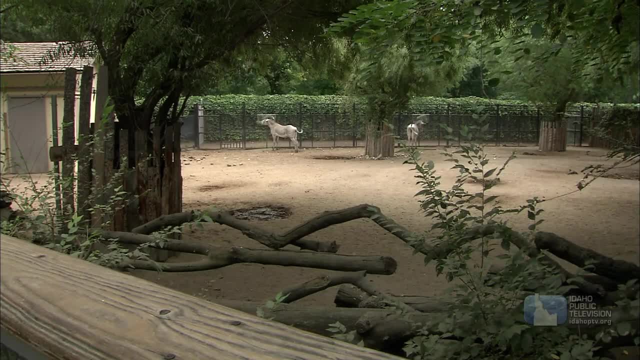 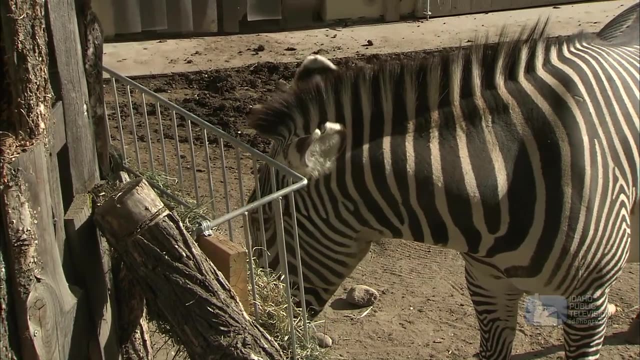 Their belly is all white Plain. zebras and other subspecies will have slightly different patterns And zebra stripes are like our fingerprints. They're different for every individual animal And we have Grevy's zebra here at the zoo because they are the closest living relative to the Idaho state fossil, the Hagerman horse. 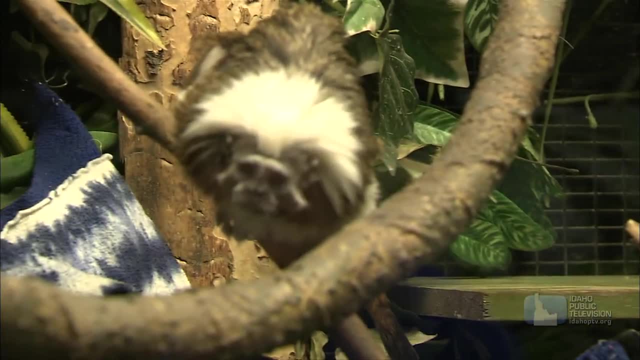 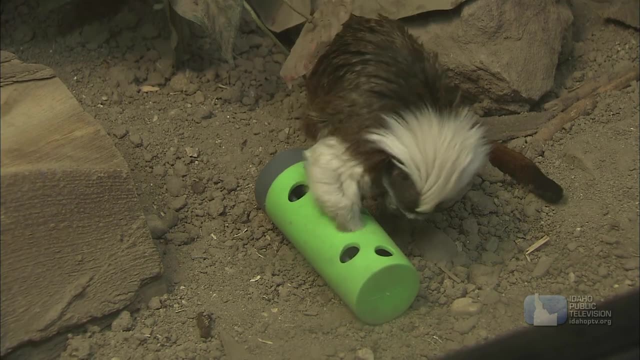 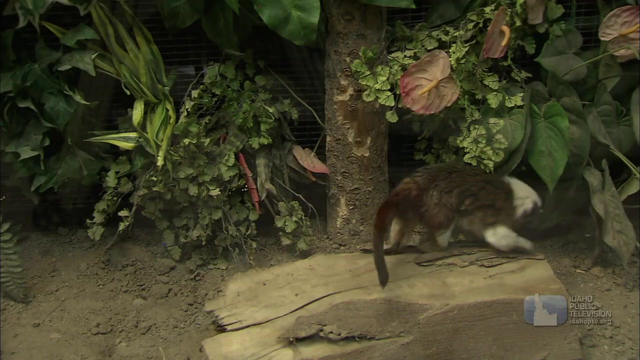 So this is Sarita. She is a cotton-top tamarin And she is a critically endangered primate from South America, predominantly Colombia, And they are a favorite here at the zoo, And they're mostly threatened for habitat loss and people catching them for the pet trade and also for medical research. 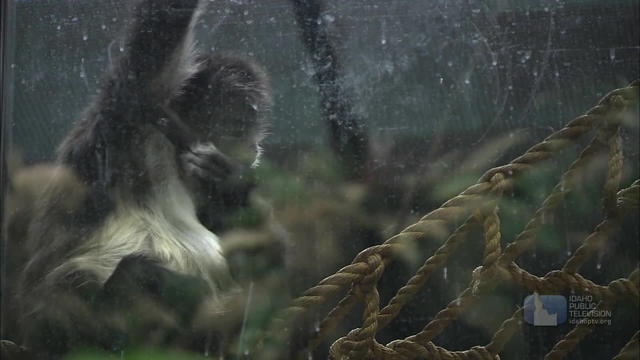 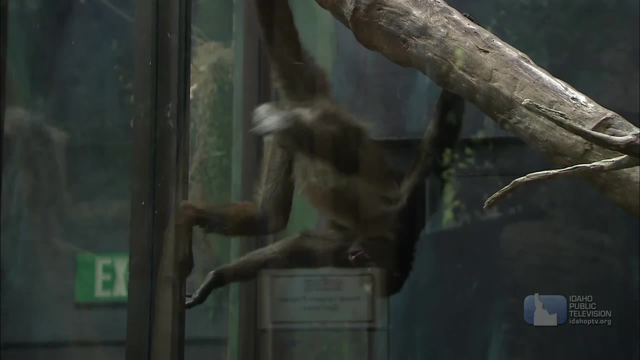 So these are black-handed spider monkeys- This is Elvis and Sarah- And they are found in Central and South America And they're really cool species because they have a prehensile tail, which means that they can use their tail kind of as another arm or leg. 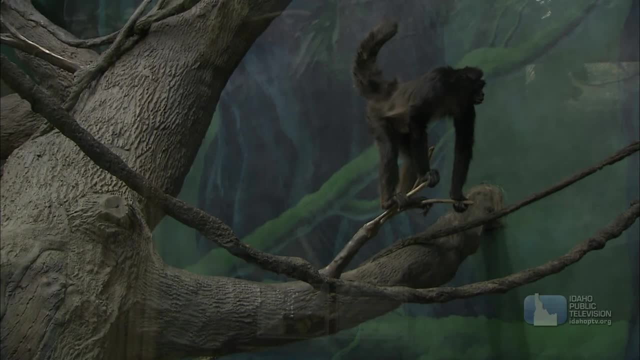 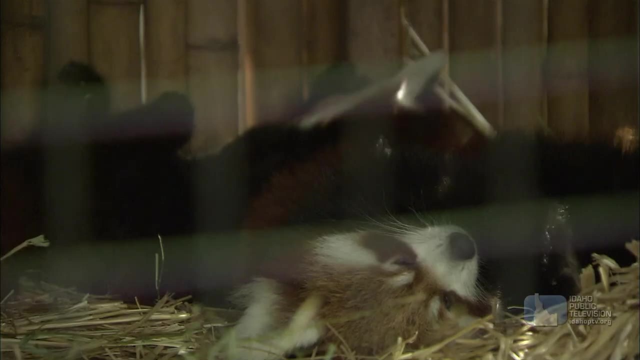 and they can use it to grab onto things when they swing through the trees and brachiate, And these guys are endangered as well, mostly due to deforestation and habitat loss. These are our red pandas, And the two you're looking at right now are our red panda cubs. 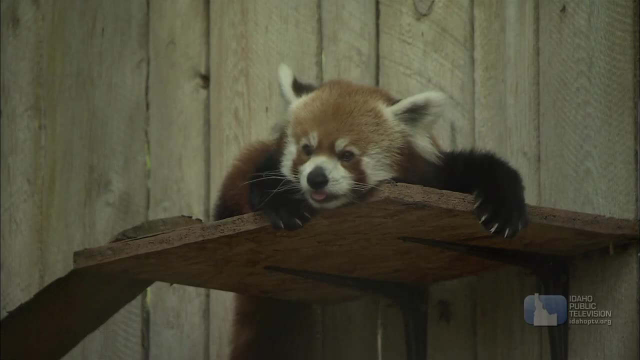 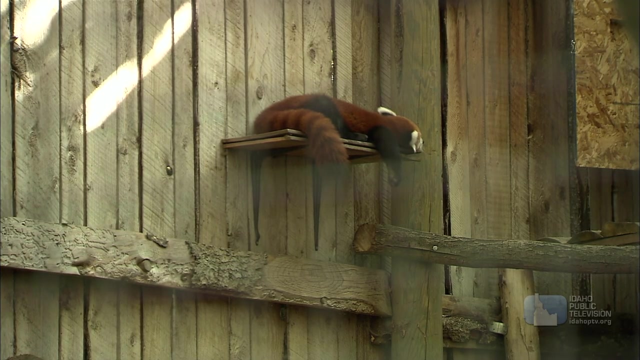 that were born here at the zoo this summer. So we have mom and dad and these two boys, And they are a highly endangered species found in Asia or in China, Nepal, India, high altitudes. They're not related to pandas. 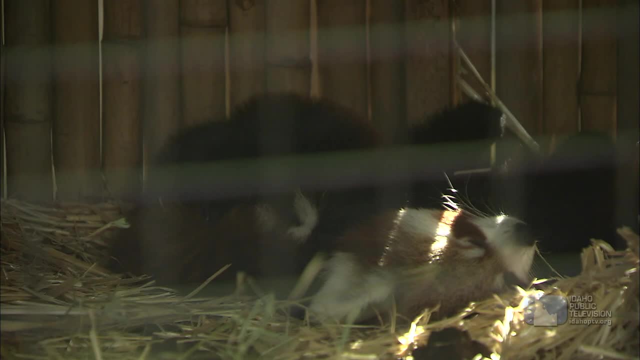 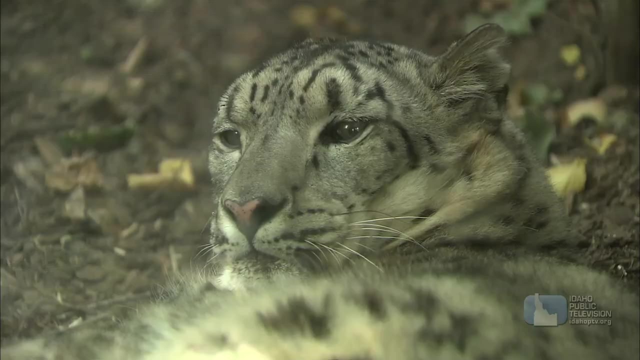 but they eat bamboo, So that panda means bamboo eater, And they are mostly threatened due to habitat loss, the pet trade and other human encroachment. This is Tashi. He's our male snow leopard here at the zoo, And we also have a female Kibita. 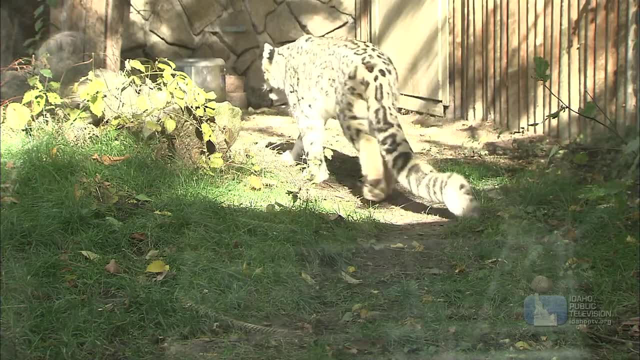 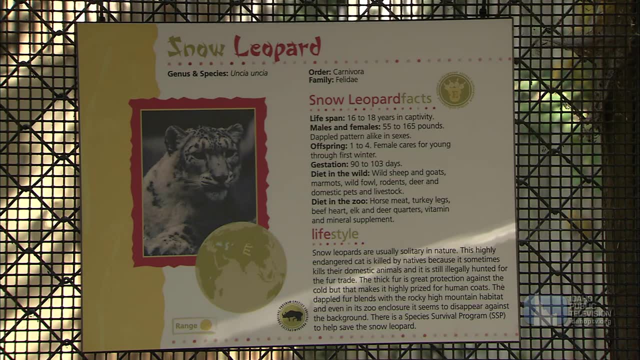 And snow leopards are a really cool cat. They're found in high altitude mountain ranges in Asia And it's really hard for scientists to know how many there are left in the wild because they're really hard to find. So they are critically endangered. There's probably less than 5,000 of them And the two we have here are paired up as part of our species survival plan to hopefully mate here at the zoo and produce some cubs and help keep their species alive. You can help save these and other endangered animals by visiting Zoo Boise. 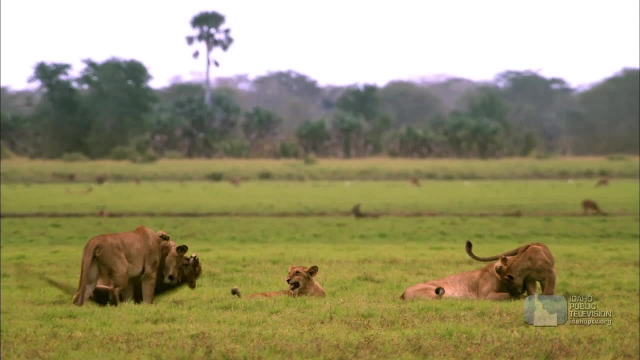 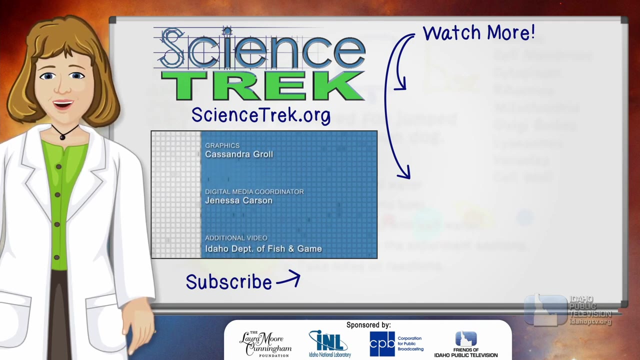 Part of your entrance fee goes to a conservation program saving animals in the wild. If you want to learn more, head to the Science Trek website or check our related videos. And if you like Science Trek, be sure to click the subscribe button to catch our newest videos.